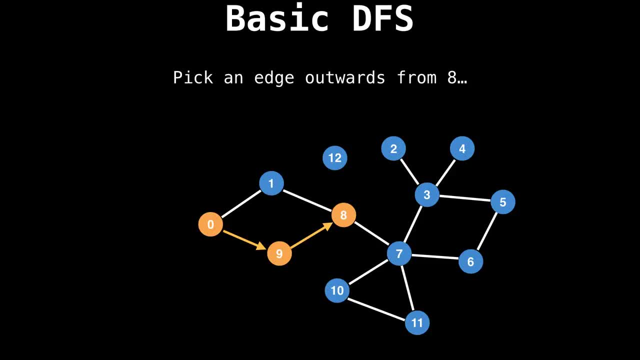 at node eight arbitrarily pick an edge. So we're going to go outwards to node seven, node seven. we have plenty of edges to choose from, So let's go to node 10, node 10 to node 11, and 11 to seven. So we don't want to revisit. 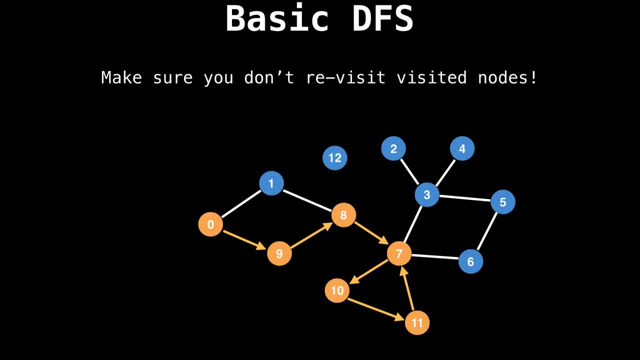 already visited nodes or nodes that are currently being visited. So we have to backtrack. To indicate backtracking, I'm going to label edges and nodes as gray, So backtrack all the way back to node seven. So we're not finished exploring node seven, Because we're going 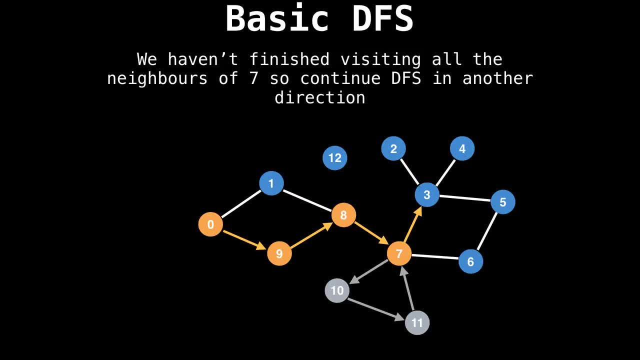 to go to node eight because there are still edges to be picked. So I'm going to go to node three And node three. I'm going to go to node two. no two is a dead end, So we backtrack, then go to node four. node four is also a dead end, So backtrack from node four back. 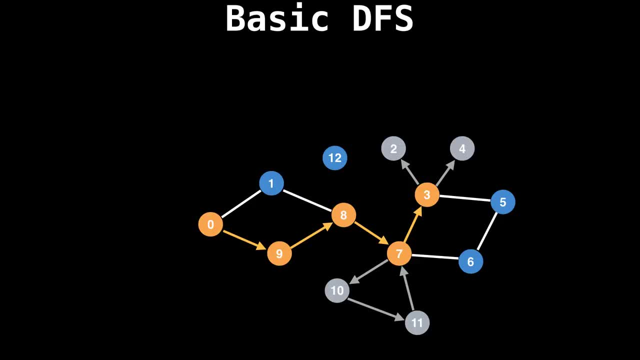 to node three, then pick node threes last edge to go to node five. five to six and six to seven. Can't go to seven because we're visiting seven currently, So backtrack all the way back to node eight From node eight. we still need to visit its. 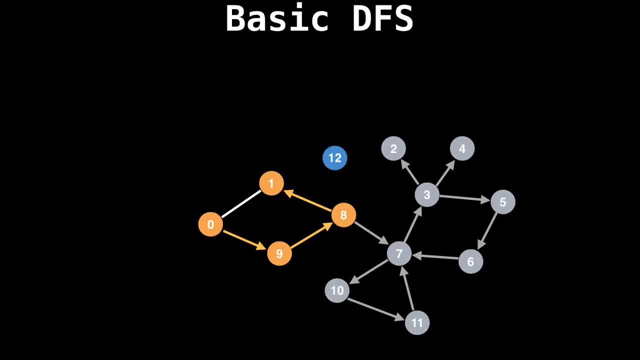 last edge, which goes to node one, node one, back to node zero. we can't go to node zero because we're currently exploring it- then backtrack all the way to zero, which completes our depth first search traversal of this graph. So this was one particular depth first search. 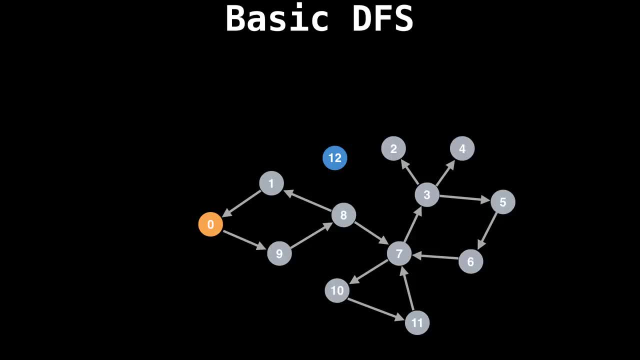 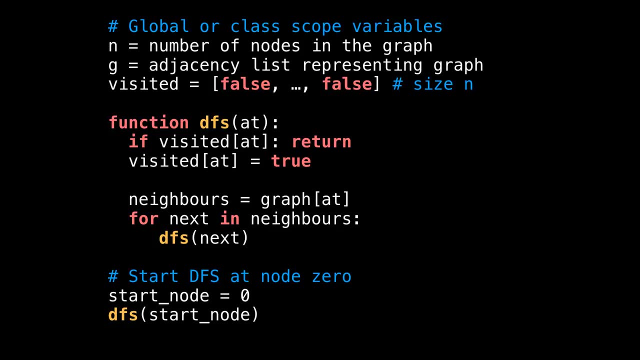 traversal, But, as you saw, it could have gone a lot of different ways. So now let's look at some pseudocode for this depth first search to get a deeper understanding of how it works. The first thing we'll need to do is initialize these three variables, which are: n- the number, 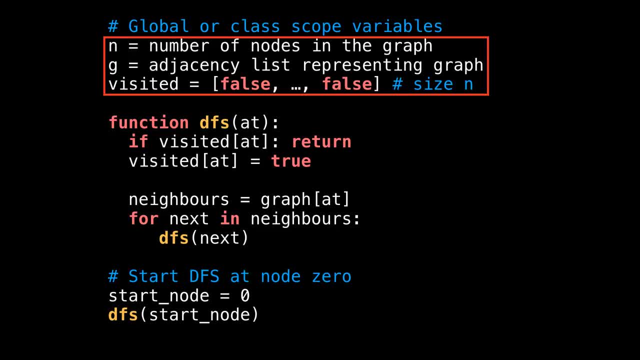 of nodes in our graph g- the adjacency list representing the graph- And visited a Boolean array containing true or false at index i, depending on whether or not node i has been visited In the beginning. this array should have all false values because we have not visited any nodes in the graph. Once that is set up, At the bottom I define: 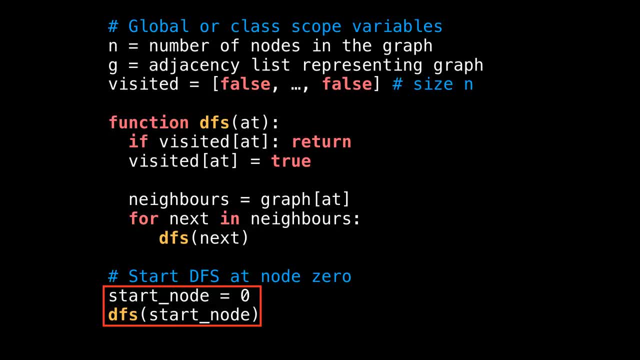 our starting node to be node zero and then call the depth first search method to do the exploration. The depth first search itself has a value of zero, So we're going to call it the depth first search method to do the exploration, The depth first search itself. 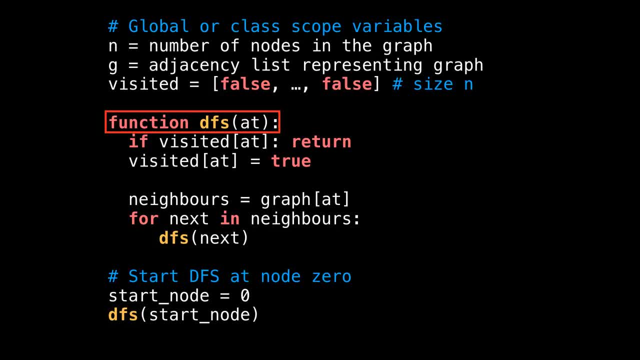 has one argument. the current node we are at, which I have conveniently named at this method, is recursive, So I checked the base case, which is whether we have already visited this node. If so, we have no business here and can return. Otherwise, let's visit this. 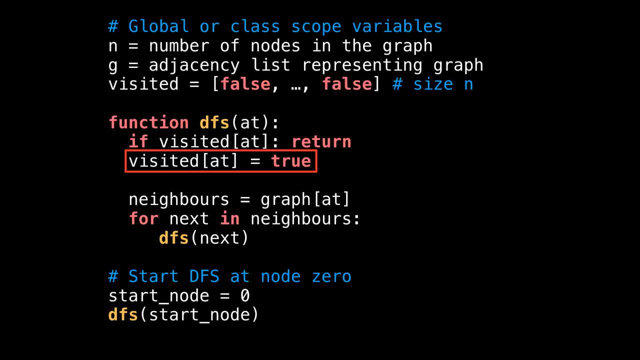 node by marking it as true and exploring all of its neighbors. To explore all the neighbors of the node, reach into the adjacency list and pull Out all the neighbors of this node and explore them depth first by looping over each and recursively calling the depth first search method. And that's all: a depth first search. 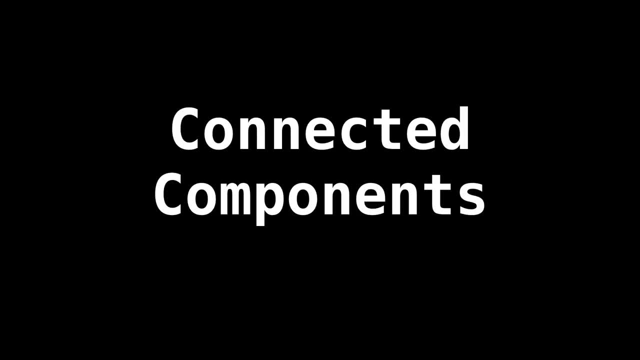 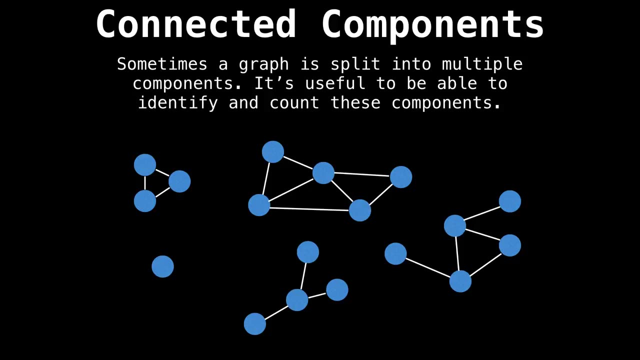 really is. in a nutshell, Let's look at another simple use case for depth for search. I want to discuss finding connected components in a graph. First, let's understand what we mean by connected component. Sometimes the graph is split into multiple disjoint components And it's useful to be able to identify and count these components. 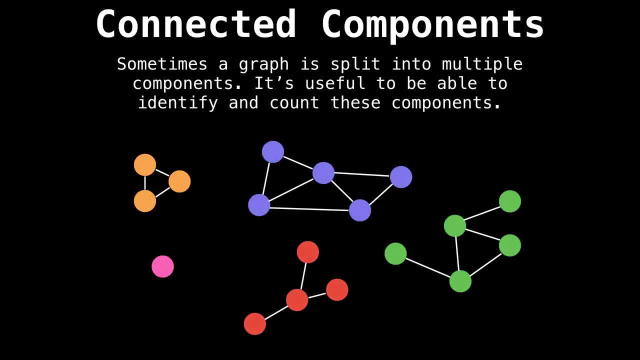 One way to identify these components might be to color them so we can tell them apart. But what does coloring nodes really mean to a computer? coloring nodes is equivalent to labeling each node in a component with the same ID value. For example, every node. 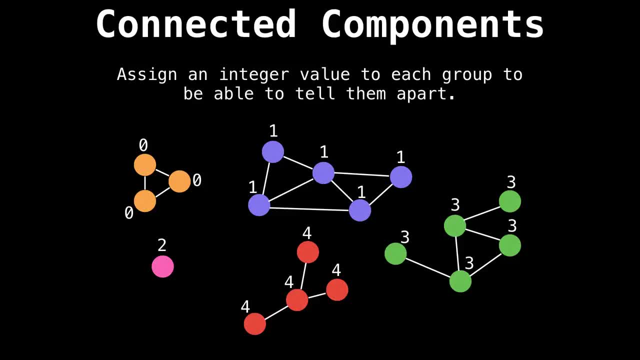 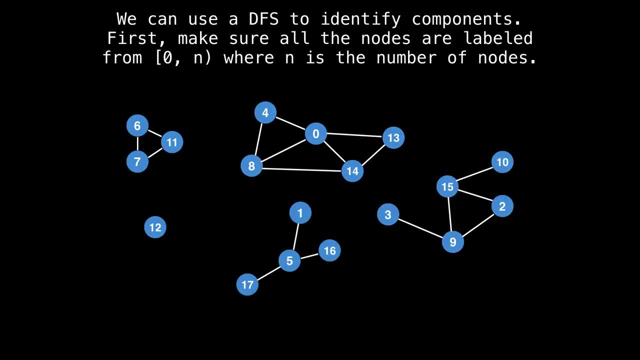 in the purple component gets an ID of one And every node in the green component gets an ID of three. We can use a depth first search to identify components this way. First, make sure all the nodes are labeled from zero to n, non inclusive, where n is the number. 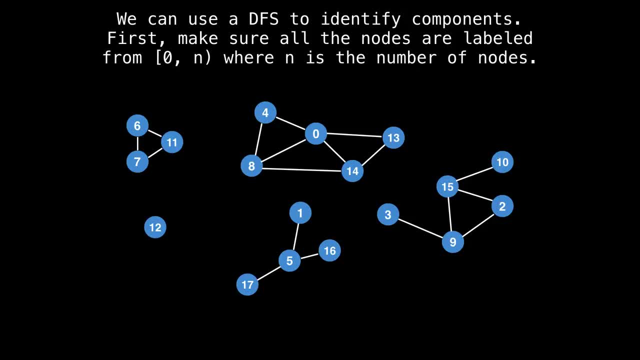 of nodes. The basic algorithm is to start a depth first search at every node, except if that node has already been visited, and mark all reachable nodes as being part of the same component using the same ID. So if we start at 0,, 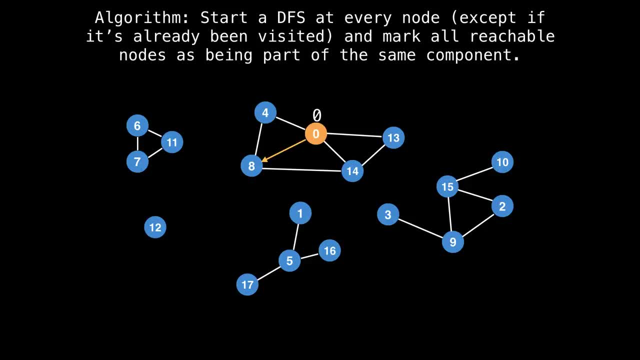 node zero. then we do a depth first search here And then every node in this component gets an ID of zero. So go to eight: given an ID of 014, gets 013. Also label it with a zero, then backtrack, like you do a depth first search, then explore node four, give: 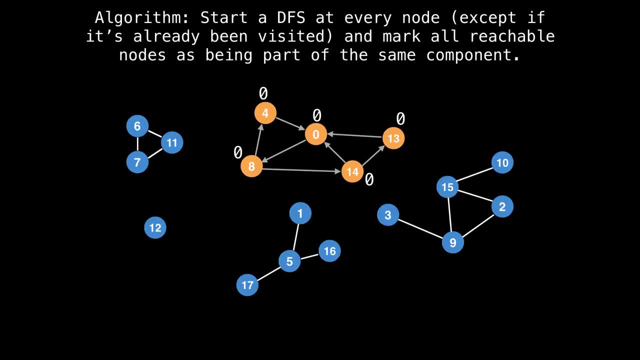 it an ID of zero and then finish exploring that component and then move on to the next node in order. So go to node one. next then node one. sorry, depth first search there. So go to node five. label it with a 15, goes to 17,. label it with a one backtrack, go to 16.. Also label it. 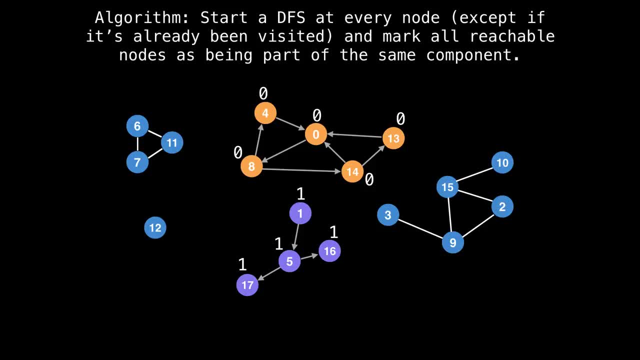 with a one, we're finished exploring this component. then we would go on to node two, wherever node two is then explore that component, then node three explore node threes component, unless node three has already been visited, and so on. 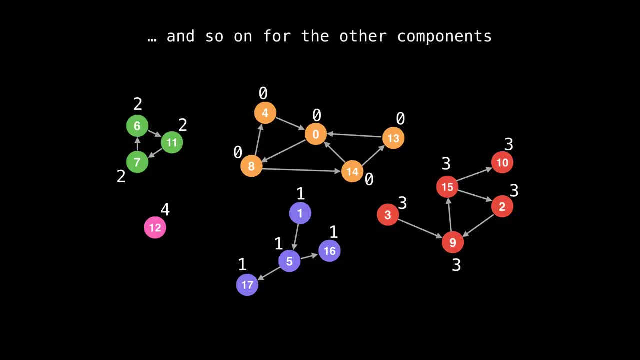 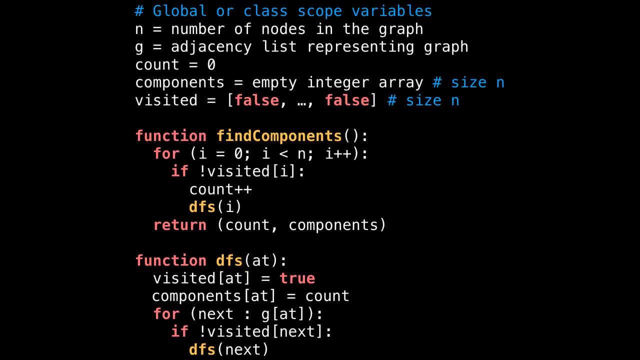 So we do this for every component And eventually we get to label all the components And we use a depth first search to do that. Awesome. So that's how we find connected components using a depth first search. Now let's look at some pseudocode for how we do this First, 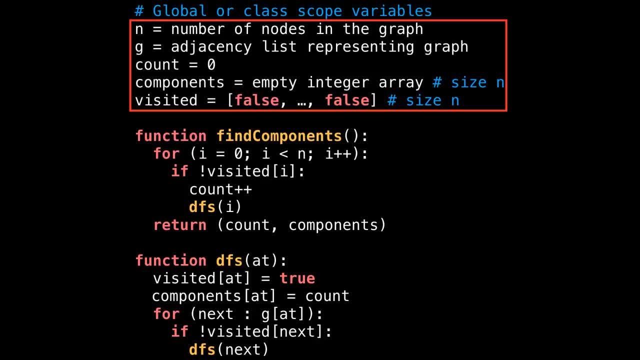 we'll need a couple of things. We'll need everything from the previous code. we looked at So n and the number of nodes in our graph g, our jc najn chocolates and our visited Array, your property And our history in Britainмicro. we also name this list on the 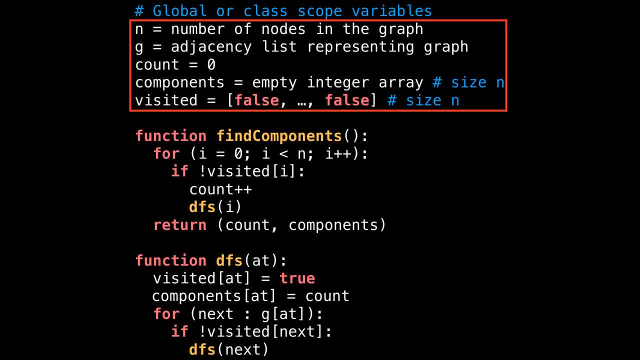 on that because we see it as For the URL, first line выб, municipality graph, bucket array. But additionally we'll also need a variable called count that tracks the number of connected components and components, an integer array that holds the integer value of which component a node belongs to. Inside the find components method we loop over every. 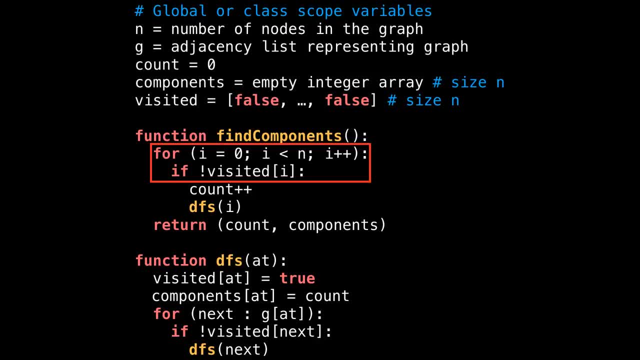 node and check if the current node has been visited or not, and then execute some logic. This depth first search variant differs slightly from the previous in that we execute a depth first search for every unvisited node. when we actually do the depth first search, we